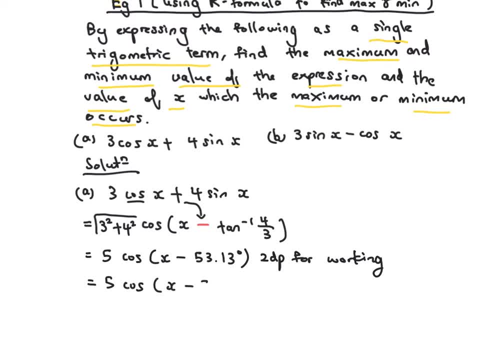 So it's 5 cos x minus 53.1.. So that is the answer for expressing the two trigonometric terms into a single trigonometric term. Now let's proceed to find the maximum and minimum value of this expression. Now we know that the cosine graph, starting from original, is equal to 0.. 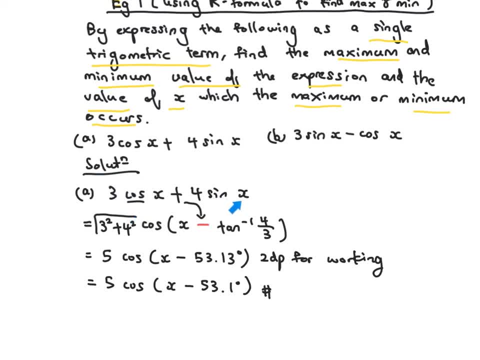 And then the product starts again ît. So what does the sin graph do? Well, the sin graph starts from, from the origin of a taper, And then makes the crest. So the sin graph actually starts from origin And then makes a descent, And then a descent. 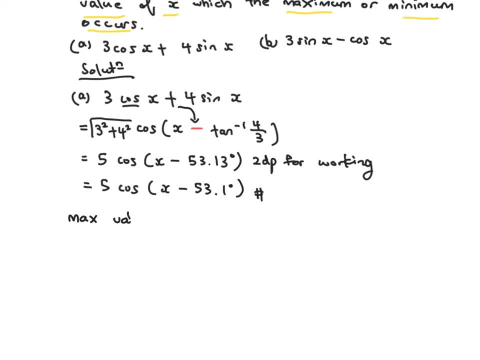 But the sin graph actually starts from origin with an descent to get the max value. So the max value is equivalent to 5 times the max value of any cosine graph, which is 1.. So it's 5, and it happens when the cosine value actually reaches. 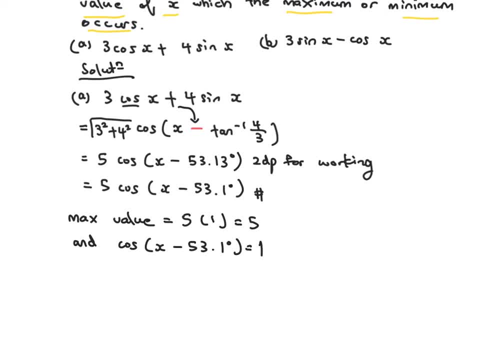 its max. The cosine value reaches its max at 1.. So looking at your cosine graph, it's like that: Now you know that it reaches 1 when x is 0, or when x is 360, which means that this angle here will be 0 degree or 360. So x minus 5, 3.1 is 0 degree or 360. Now 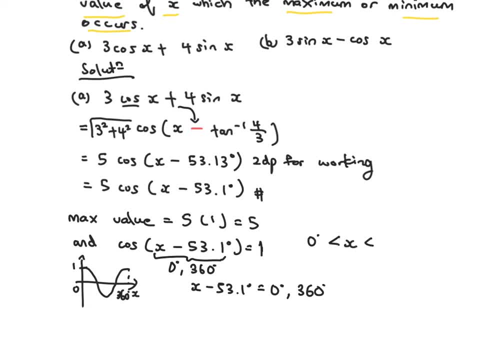 we usually solve for range of x between 0 and 360. So that means that we have a range of x between 0 and 360.. So that means that x, when you add 5,, 3.1 degree on both sides, you are going to get. 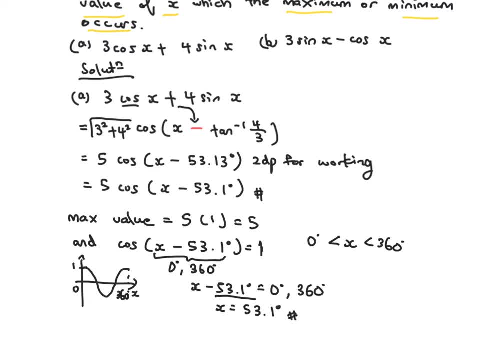 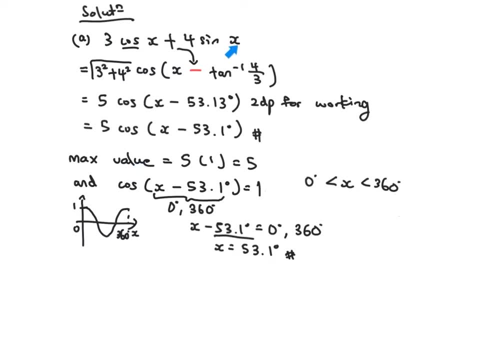 5,, 3.1, and the other angle will be rejected. So that is the answer to the question. The max value of the whole expression here is 5, and this happens when x is 5,- 3.1 degree. 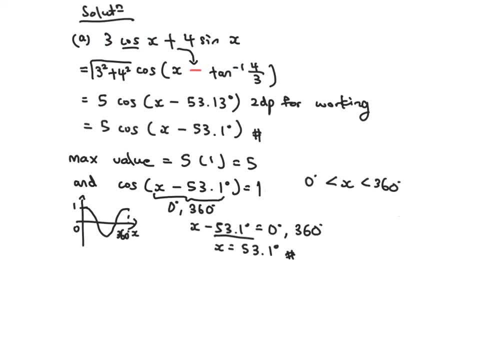 Let's proceed to get the minimum value of the whole expression by getting the minimum of this cosine term. So minimum of the value of the whole expression will be 5 times the minimum value of the cosine term, which is minus 1.. That will give me minus 5.. And the cosine value is equals to minus 1.. 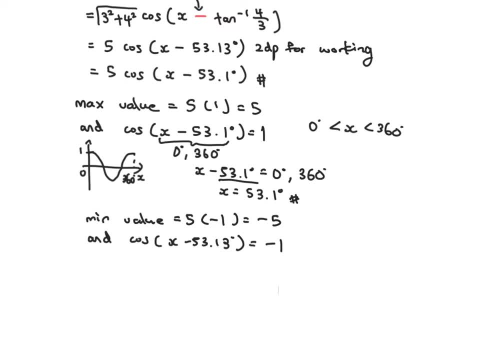 Looking at the cosine graph again, you can see that when it's minus 1, the angle is 180.. That means that this angle here will be 180. So x minus 5, 3.1, 3 is 180. So x. 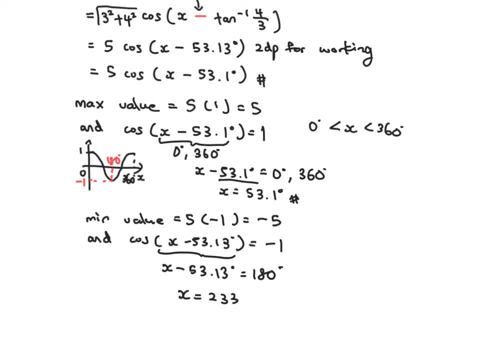 will be 2,, 3,, 3.1 degree. Now the final answer must always be 1 dp, And then the working here must always be 2 dp. So which means that previously here my this step should be 2. 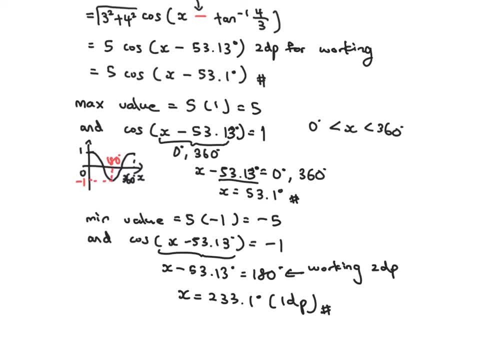 dp, 2 dp, working 2 dp, and then the final answer: 1 dp. Okay, So now we know the minimum value of the expression is minus 5, and it happens when x is 2,, 3,, 3.1.. Range of x is: 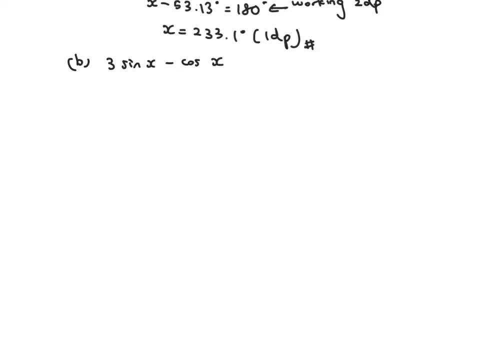 from 0 to 360.. Let's move on to part 3.. Part 3, expressing 3 sine x minus cos x as a single trigonometric term. Since sine is the first term, we will have to use the sine function And the number in front is given. 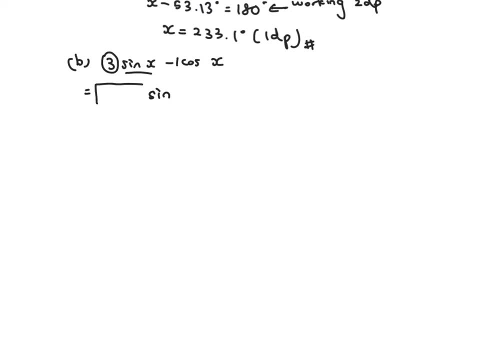 by square root of this number square and the number here square, ignoring the sine, So it's 3 square plus 1 square. Since I'm using sine, I will have to copy the sine function in the question, The minus place over here And then tangent inverse second number over. 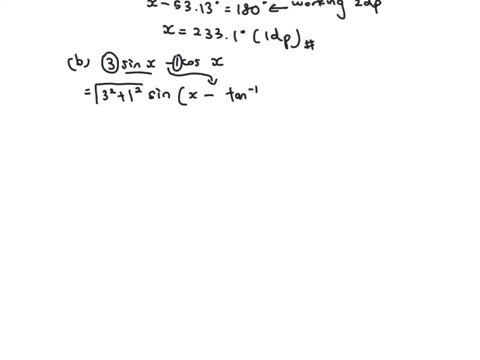 the first number, ignoring the sine again, So it's 1 third. Then, evaluating the answer, I get root 10 sine x minus 18.43, working 2 dp. And then, after that final answer, I'll get 1 dp sine x minus 18.4 degree. So this is my answer. Now I go ahead to find the max. 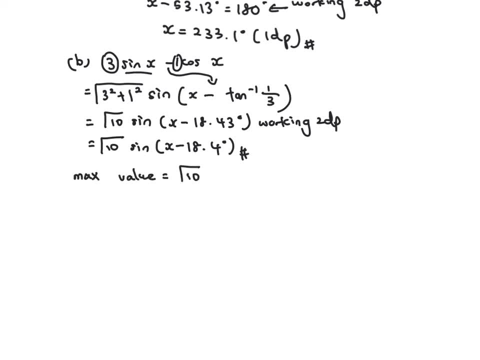 value of the whole expression will be root 10.. The max value of this is equal to the max value of this. Okay, Max value of the sine graph is 1.. So root 10 times 1, which is root 10.. 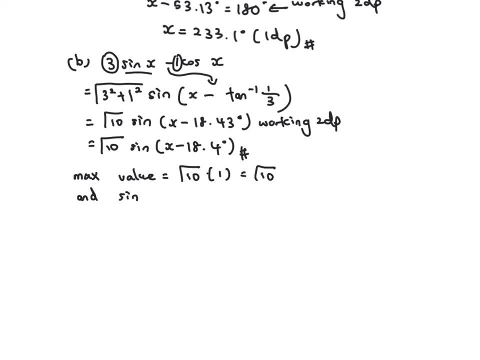 And your curve is 1.. And your curve is 1.. I friend your sign value 3 times or y times, So don't worry. and because the value of this is same as the example, you need to do 1 again to get your value. 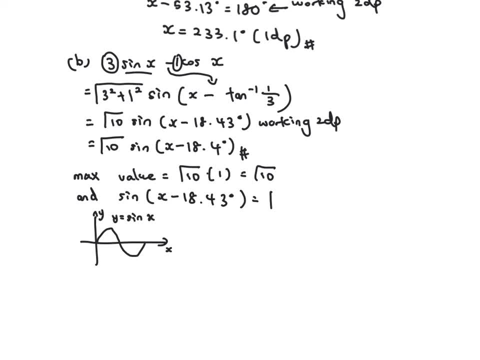 And this is the maximum value of the value of the crux And the strength of the torque is 0.. The shaft is still the same to be. the maximum- Excuse me Stop- is 1.. So this must be 90.. So which means that your x value will be 108.4.. Final answer round up to: 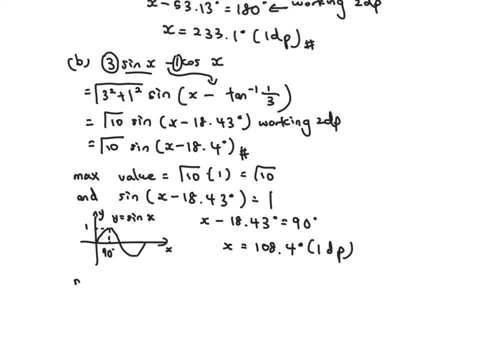 1 dp. Let's proceed with the minimum value. The minimum value of the whole expression will be root 10 times the minimum value of the sine graph. Now you can see the minimum value of the sine graph is minus 1.. So I'm going to put: the sine value is minus 1.. So the minimum value of the 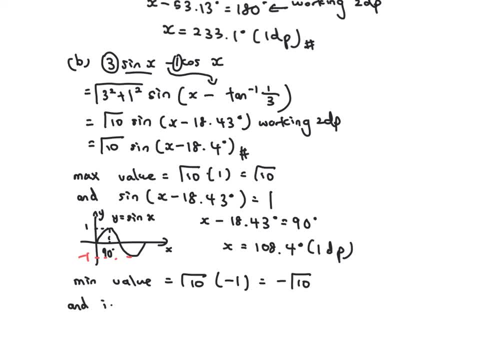 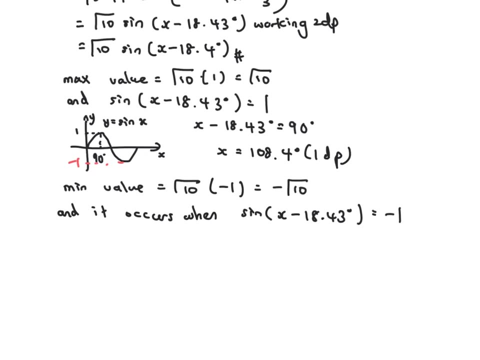 whole expression is minus root 10. And it occurs when you make your sine value as minus 1.. Looking at the graph again, when you make your sine value as minus 1, you can see that the minimum value of the whole expression is.